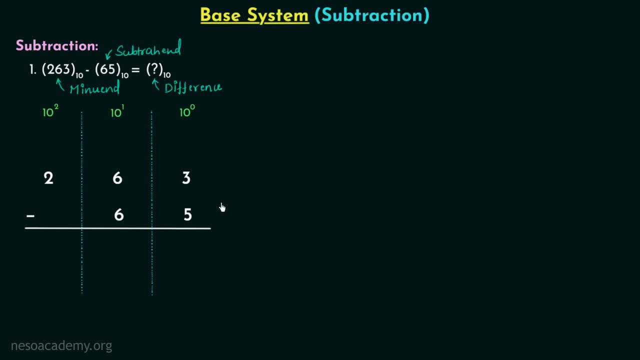 3 minus 5 will give us minus 2.. So you can see that we are getting a negative result, And the reason for this is the digit 5 is larger than the digit 3.. And whenever the digit of the subtrahend is greater than the digit of the minuend, we perform the borrowing. 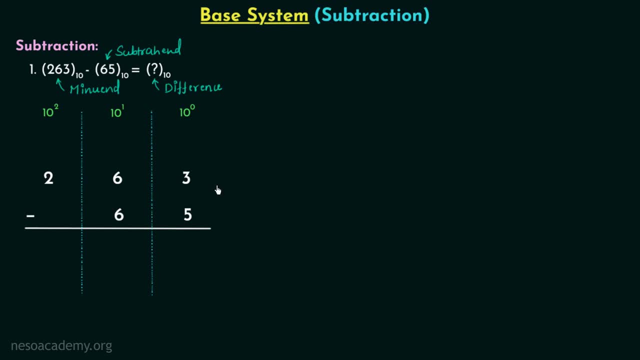 Now, what do we mean by the borrowing? Borrowing is the process in which we take the value from the digit having the higher place value And then the value taken will be added to the digit having the lower place value, And it is performed when the digit in the minuend is smaller than the digit in the subtrahend. 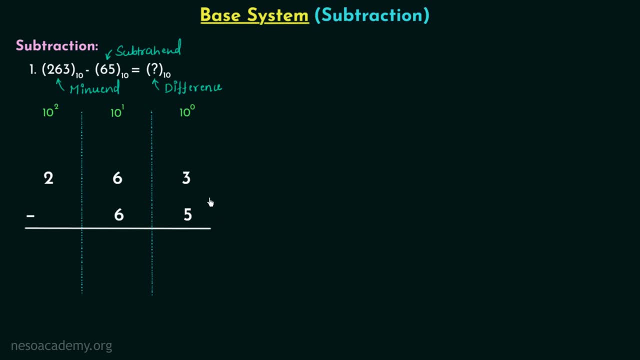 Which is happening in this case. So we are going to take the borrow from digit 6, which is having the higher place value than digit 3.. Now digit 6 will give a value to digit 3 in order to make it larger than 5.. 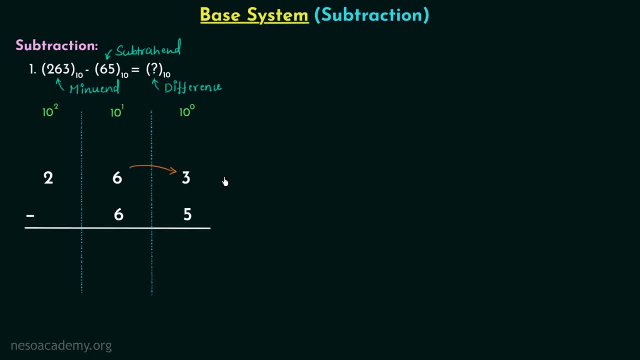 And how much 6 is going to give to 3?? It will give 1 to 3.. And 1,, which is having the place value 10 raised to power 3.. And 1,, which is having the place value 10 raised to power 3.. 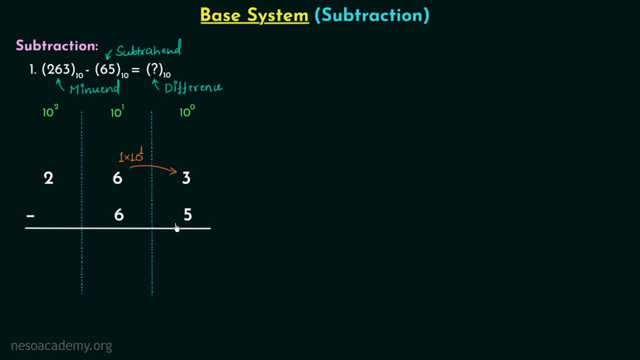 And 1,. when goes to this column, it will be written as 10 multiplied to 10 power 0. So 6 gave 1, which, when came to this column, is written as 10.. We already understand how the digits are written, as per the place values. 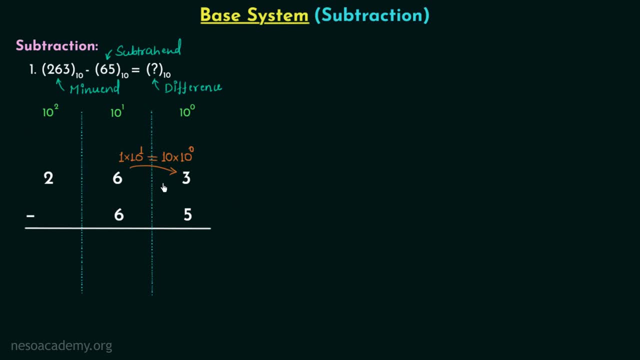 And now we will move on to the next step, in which we will add digit 3 to 10, which is having the place value 10 raised to power 3.. So digit 3 is taken from 6.. So 3 plus 10 is equal to 13.. 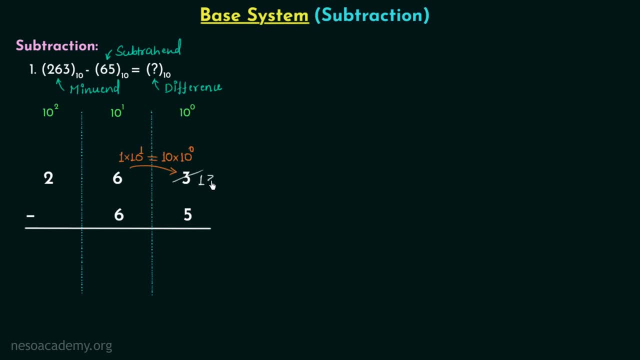 And now, instead of 3, we will have 13.. And here, instead of 6, we will have 5.. And now we can subtract 5 from 13 and it will give us 8.. And after this we will move on to subtract the digit of the subtrahend at 10th place. 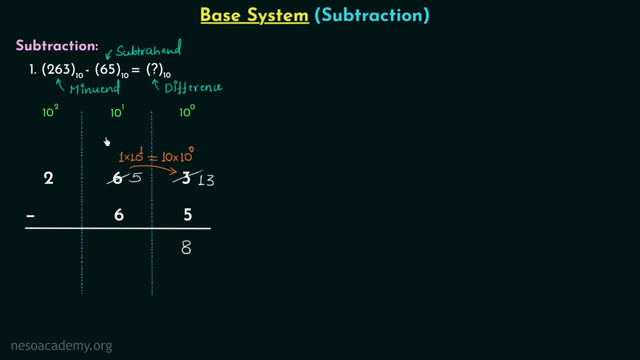 from the digit of the minuend at 10th place. 5 minus 6 will give us minus 1, and again we have a situation in which the digit of subtrahand is greater than the digit of minuend, and again we have to perform the borrowing, and this time 5. 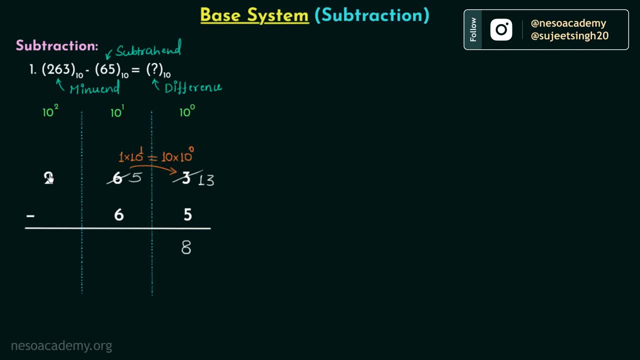 which is at 10th place, will take the borrow from 2, which is at 100th place. So 2 will give the borrow to 6 and how much borrow it will give. It will give 1 again and this 1 has the place value. 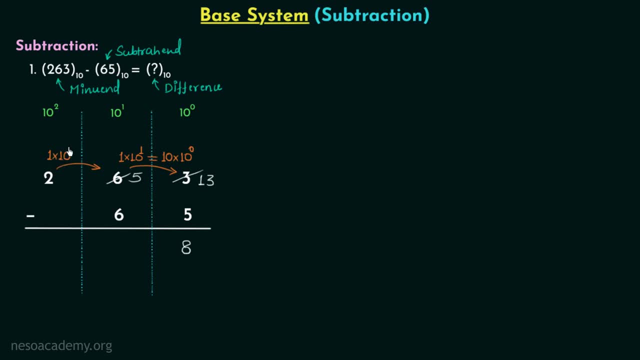 10 raised to power 2.. So we have 1 multiplied to 10 raised to power 2, and when this 1 is written at 10th place, it will be 10 multiplied to 10, power 1.. So you can see that 5 is getting 10. 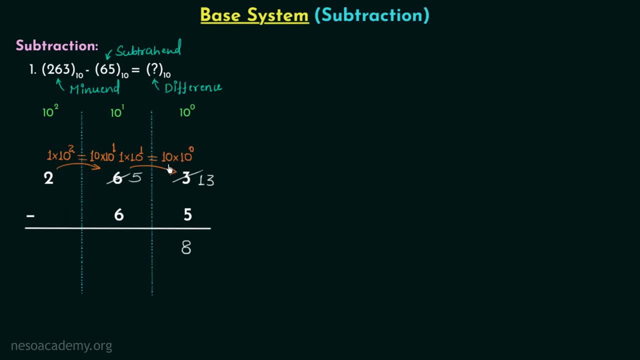 after borrowing like, 3 was getting 10.. So from here we can draw a very important conclusion. We can draw the conclusion that whenever borrow happens, the digit borrowing will get the value equal to the base of the number system. In the first case, when 3 borrowed from 6, it got value equal to 10, which is the base of. 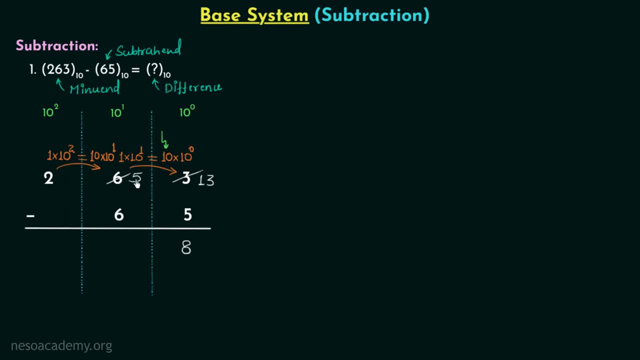 decimal number system. and in the second case, when 5 borrowed from 2, it again got 10, which is the base of decimal number system. So every time when the borrowing is happening, the amount borrowed is equal to the base of the number system. So I can write: the borrow is always going. 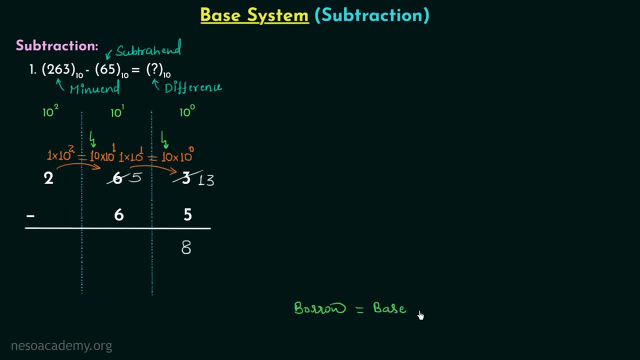 to be equal to the base of the number system and remember, 1 will be deducted from the digit giving the borrow, always in all the number systems, And so from now on, we are only going to follow this and not get involved in the calculations, keeping the place values in mind. 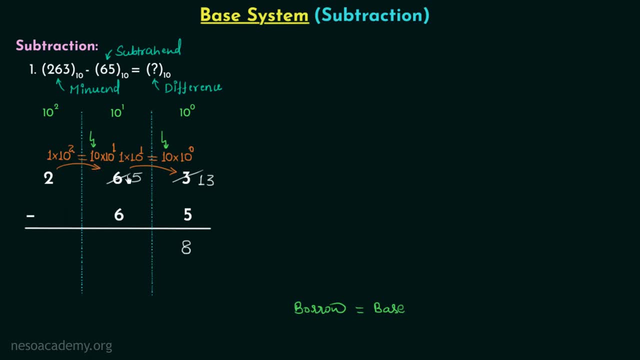 So let us continue our subtraction: 10 plus 5 is equal to 15.. So in place of 5, we will have 15 now, and here, in place of 2, we will have 1.. 15 minus 6 is equal to 9.. And this 1 is subtracted from, while 1 comes out rhetorically. The second means 15 minus 6 is equal to 9.. And this 1 is now subtracted from 5.. So here, in place of 2, we have now subtracted from this 1.. 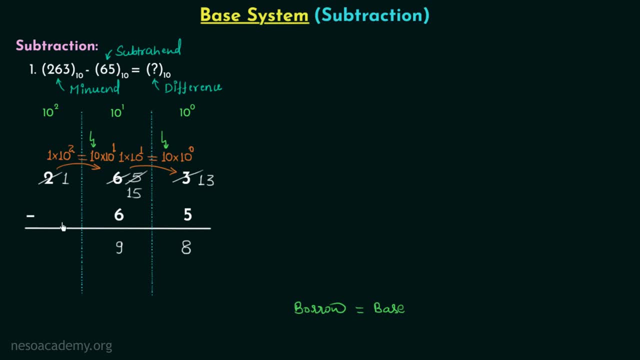 And here, in place of 2, we have now subtracted from this 1.. And this 1 is now subtracted from this 1.. is now subtracted by zero. We have zero here, which we usually do not write, So one minus. 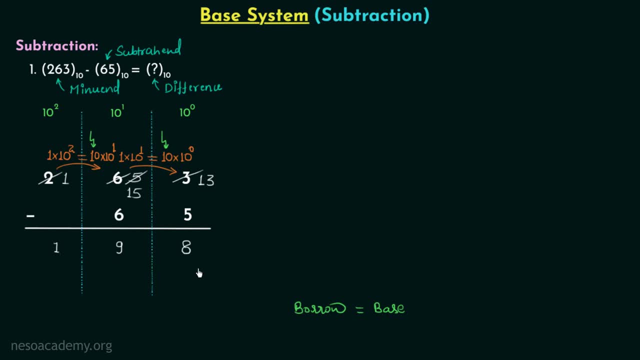 zero is equal to one, So one nine eight in decimal is the answer or the difference of this subtraction. So I hope you now understand the entire process of subtraction in a given number system and you also understand why the borrow will be equal to base. 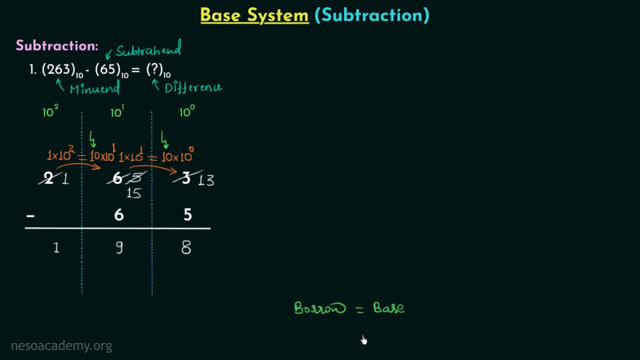 of the number system, and this we are going to use in other number systems directly. So let us move on to our second question. In this we want to subtract one one in binary from one zero zero in binary and we want to note down the result in binary. 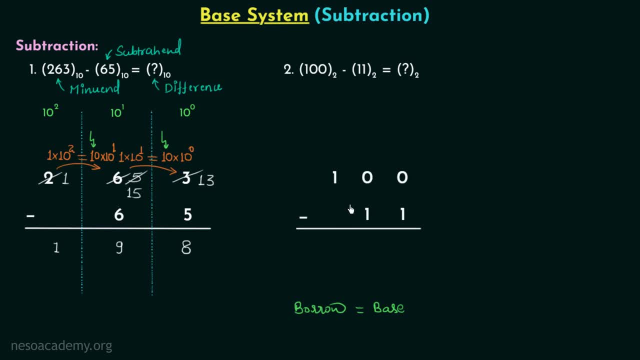 So the minuend is one zero zero and the subtrahend is one one, and after placing the digits as per the place values, we can start the subtraction process. zero minus one. the digit of the minuend is smaller than the digit of the. 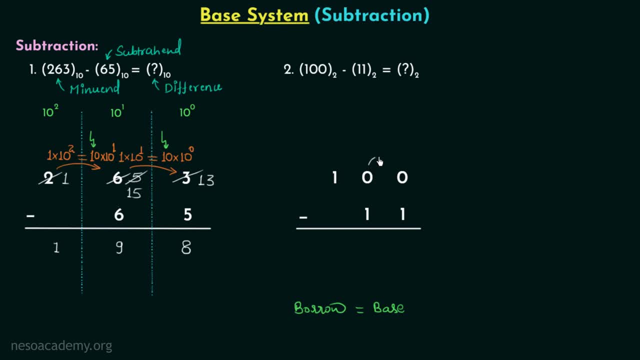 subtrahend, so we will take the borrow. zero cannot give the borrow, so zero itself has to take the borrow first, zero. when take the borrow from one, the value of the borrow will be two, because two is the base and we know the borrow value is equal to the base of. 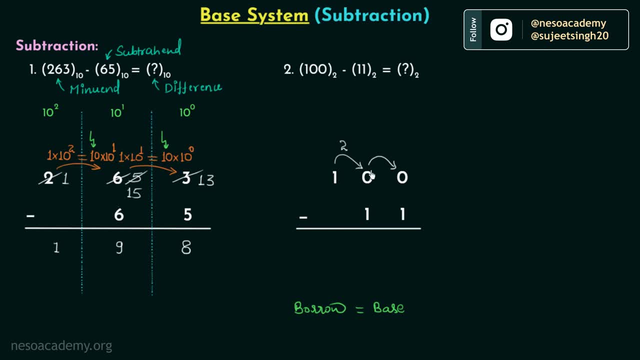 the number system. so one gave two to zero. two plus zero is equal to two. so now we have two in place of zero and we will have zero in place of one. now this two will give the borrow to zero and the borrow will be equal to two. so 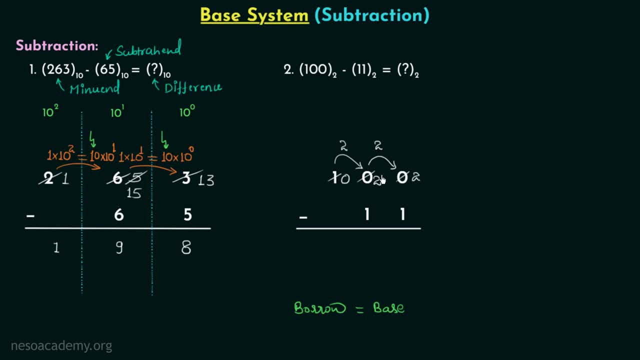 two plus zero will give us two. here and here we will have one. now we can perform the subtraction process: two minus one is equal to one, one minus one is equal to zero and zero minus zero is equal to zero. so when we subtract one, one in binary from: